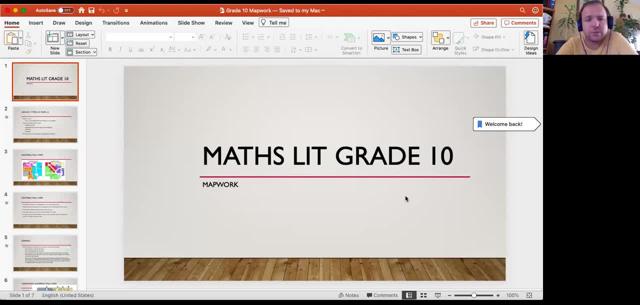 types of maps you can get in math literacy and also how to deal with some basic questions regarding each one. Now, the basic questions you're going to deal with mainly are going to revolve around how to explain to get from one place to another, All right, and also you're. 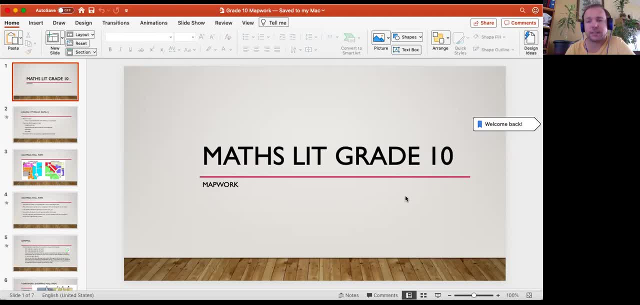 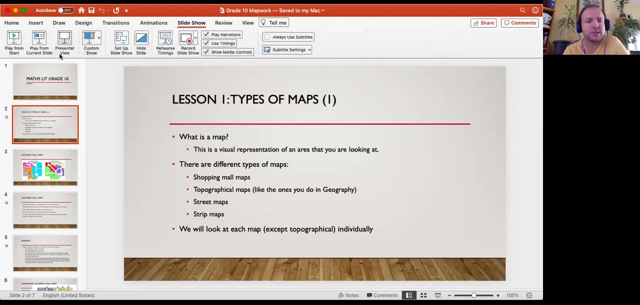 going to deal with a lot of basics like, for example, calculating distances in terms of certain maps and working out the different directions between different points on the map. All right, so let's just quickly go through it. What is a map? Let me just put this on my slide. 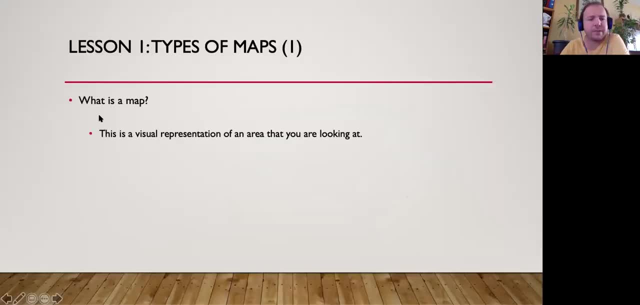 All right, so what is a map? This is basically a visual representation of an area that you're looking at. So now, if I want to talk about, let's say, a map of a school, I'm just simply saying: how would the school look like from above? All right, now we're going to basically look at 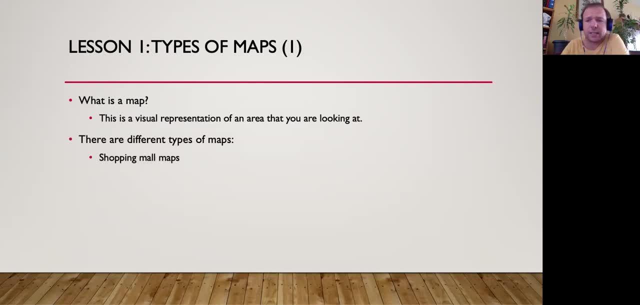 different types of maps Right now. the one we're going to look at now is on shopping mall maps. Now, it's those maps that you see when you come into the shopping mall to show where to go to for each shop. All right, you get the ones in geography, called topographical maps. Now 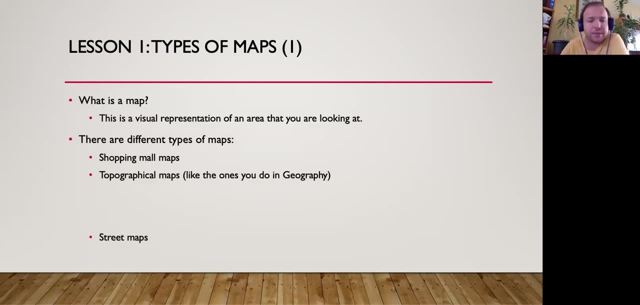 we're not going to worry about those ones. in maths literacy You deal with street maps and then also what's known as strip maps. All right now, strip maps are simply those ones where you get an individual strip. you know it's a route from one to another, Right? sometimes I refer to 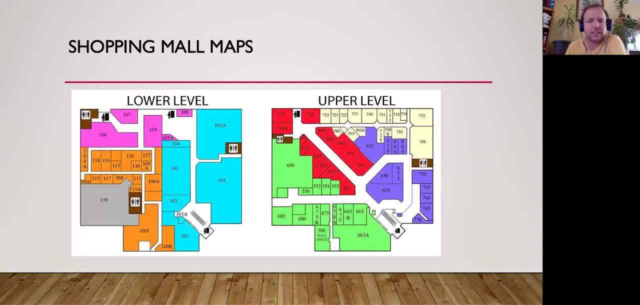 it as route maps, Right? so let's have a look at the first one: the shop Shopping mall. Now, here we're going to basically talk about a shopping mall. Now, what you need to understand about shopping mall maps is you need to identify the different components of the map. 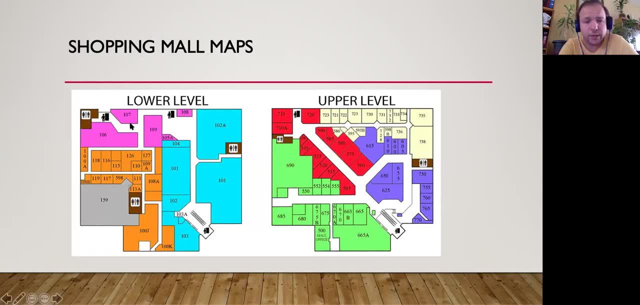 For example, if you have a look, first of all there are two levels. There's a lower level and then an upper level. All right, now what they've done is they've given you all the shop numbers, So this is shop 107.. This would be 108,, 102,, 101. 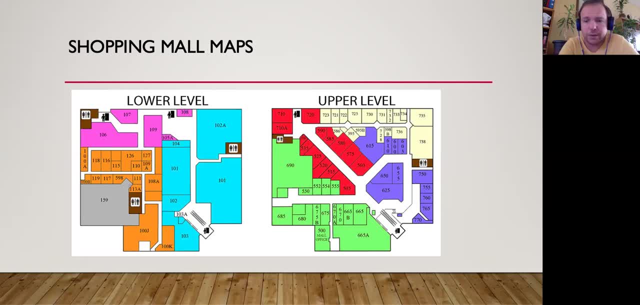 Other things that you need to worry about when it comes to maps that regards to shopping malls is sometimes you need to know where to find certain identifications. For example, here in this map, they indicate lifts to you, So this would be a lift to that side, This would be a lift to there. 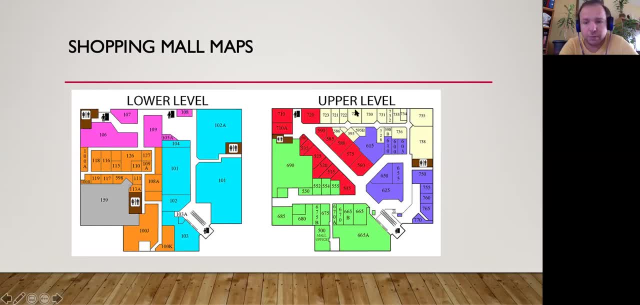 Now, this lift over here would go to probably be one of these shops over here. All right, the second one, this is a toilet, So they're showing you where the toilets are located, All right. so over here there's one, there's two, there's a three, There's basically quite a few toilets around this. 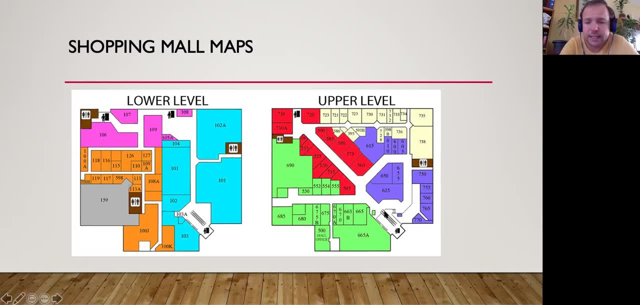 map, All right. and also they indicate the escalators as well to you by showing a line, quite a few lines, in parallel to each other. Those are the escalators. All right, now let's have a look at the questions that you're going to be expected to know in this. 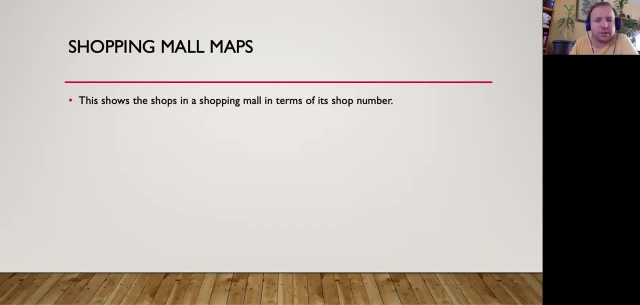 Right, the first one. This shows the shops in the shopping mall in terms of shop number. Okay, so this is the notes behind it. All right, so notice: each place had a shop number. Many other features will also be shown. If it has different levels, it will indicate it to you. 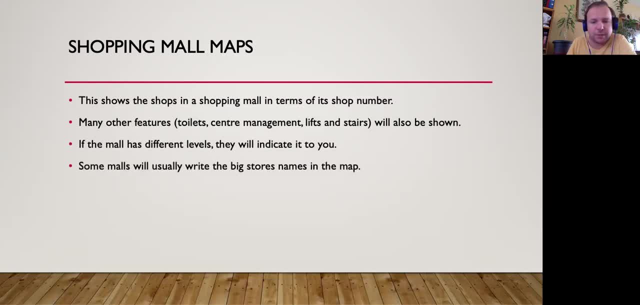 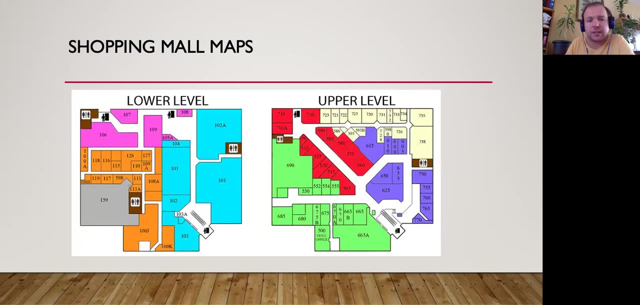 Some malls will usually write the big store names on the map, And also there are times where there are entrances involved. Now, in this example, they don't indicate the entrances to you, All right, but in the homework there will be. 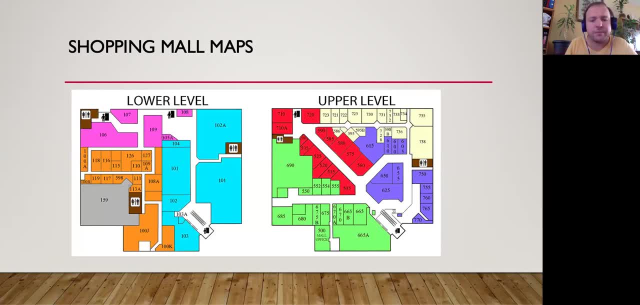 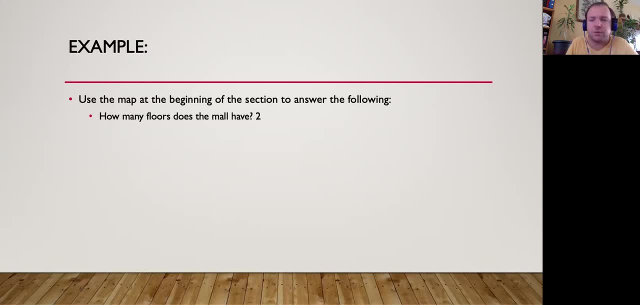 a question involving entrances. We will get to that All right example If we look at the map in the beginning: all right, there were two floors. There was an upper level, lower level, If you notice, if you go back to the toilets. all right, let's just go back quickly. 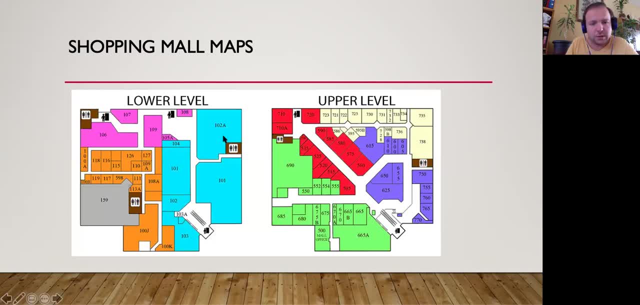 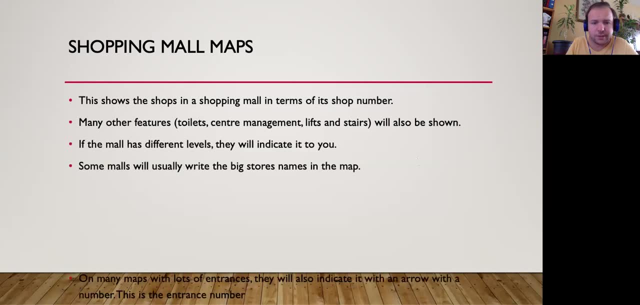 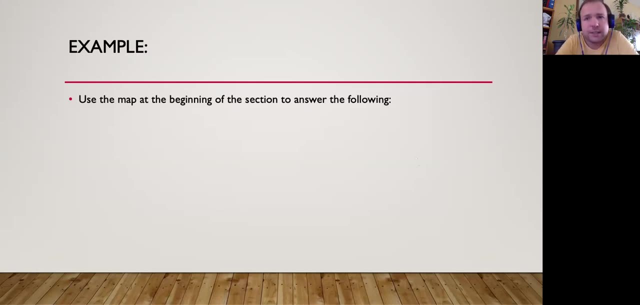 There were one, two, three, four, five toilets in this whole mall. Okay, now, sometimes they might ask you to interpret that, Say: does this have enough toilets? You could then interpret: say yes, because there's quite a lot of toilets on each floor. 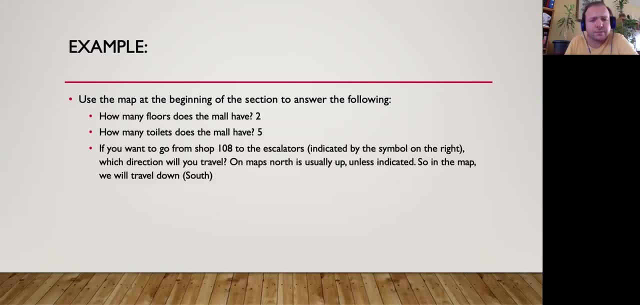 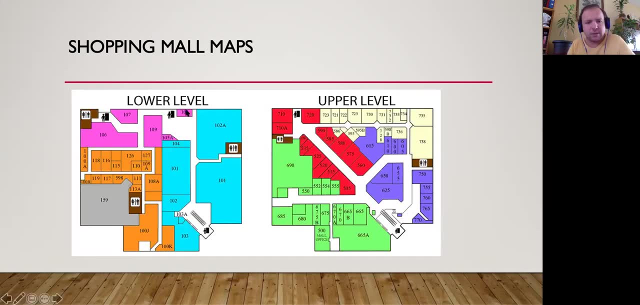 so it would be useful and they spread out. All right now, if you go from 108 to the escalator, all right, so let's say I'm going from there to the escalators. Now one thing that you need to. 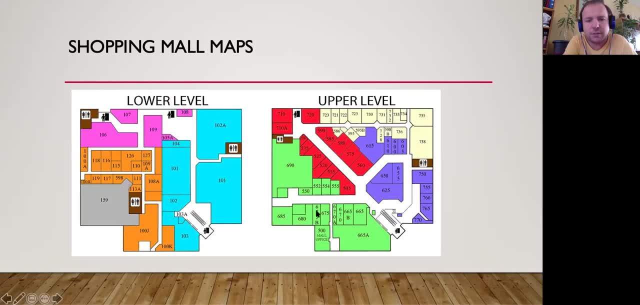 remember is that they will always, usually indicate on a map the direction right. If there's no direction mentioned to you, assume it to be north, going up, south, going down, and so on. So this would be north, this would be south, this would be east, this would be west. Same over here, North. 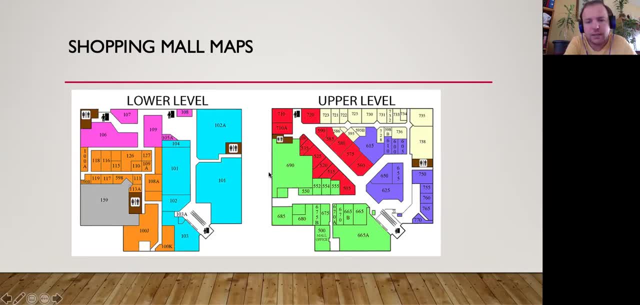 south, east And west. All right, so if we have to say, right, going from 108 to the escalators, you're going to simply travel south down the walkway to the escalators. Now, what happens is I'm going to. 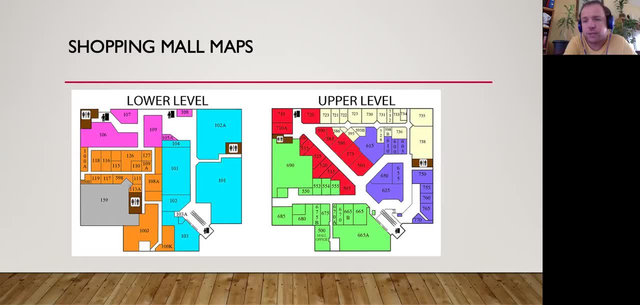 you're going to get questions where you have to basically go from one shop to another, Like, for example, in the example I've given. the question I've given there's a question involving going from this shop to this shop. Now, 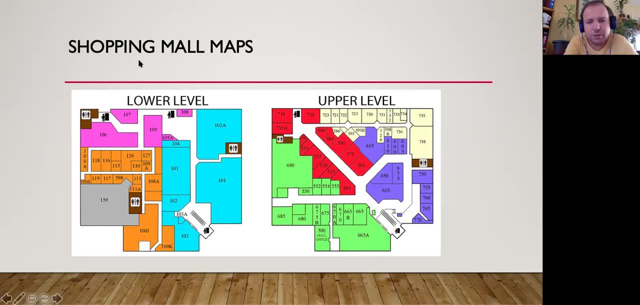 remember, to be able to get to the two shops on different levels, you have to first get to the escalators, all right, or to the lifts, all right. Now, obviously, I'm going to use the escalators up here, but you're welcome to also use the lifts if you wanted to. all right, And say travel from. 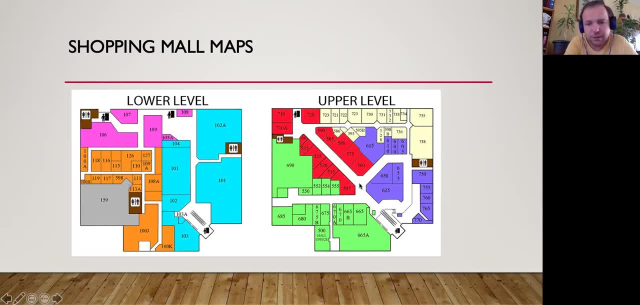 there to the lift over there and go up and then travel down. That's fine. I'm going to use it in terms of the escalators, So I'm going to go from the 108 to the escalators, go up the escalators. 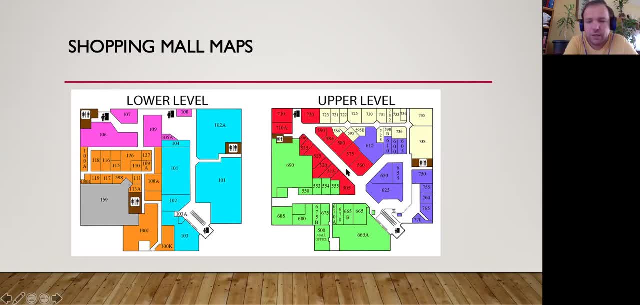 and then travel down to 505.. Now, what you need to also remember is that you need to indicate direction and also, for example, how many shops it is from the escalator. For example, if you notice over here, 505 happens to be one, two, three shops down, So you would have to say it would be your third shop. 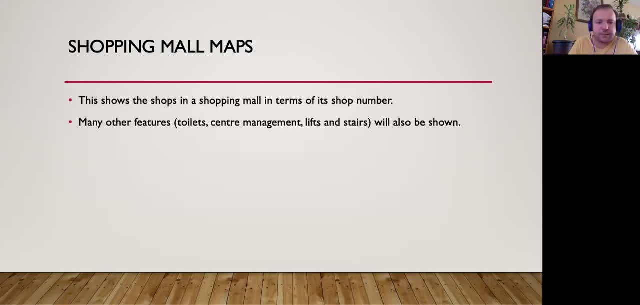 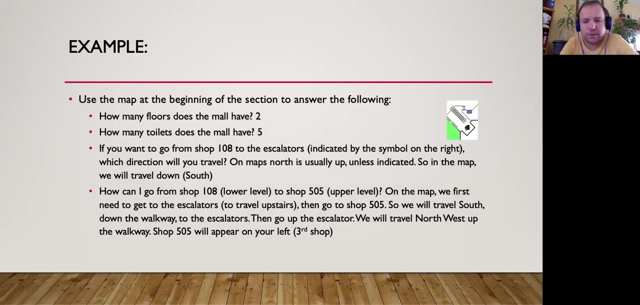 on the left. all right, And that's what I've mentioned over here. How can I travel from 108 to 505? On the map, we first need to go to the escalators, to travel upstairs, then go to 505. So we'll travel.